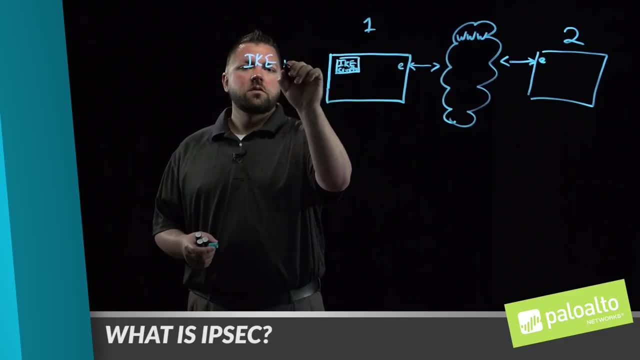 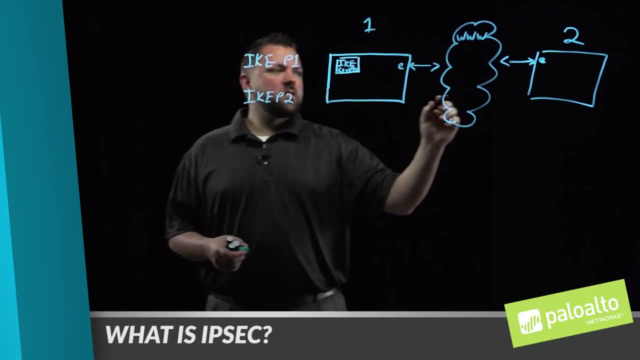 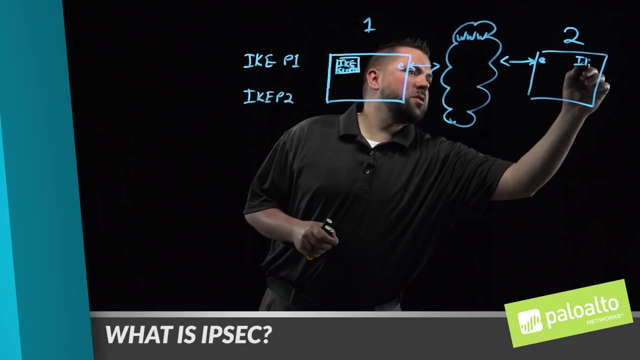 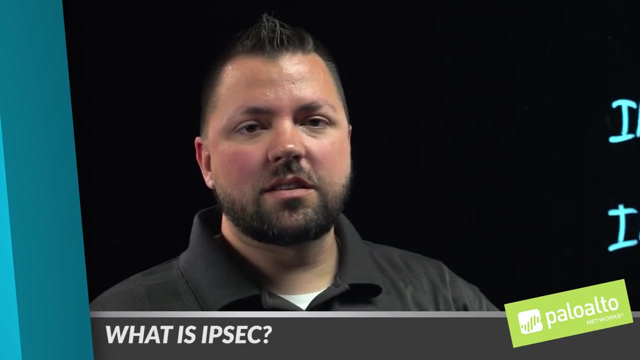 So we'll call this ikePhase1, and then down here we'll have ikePhase2.. The same ikeSettings- and that's crucial- the same ikeSettings go into the opposing firewall or the peer, so that when one wants to talk to the other, they know what each 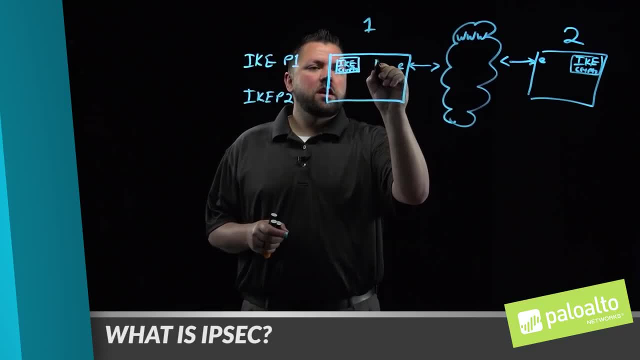 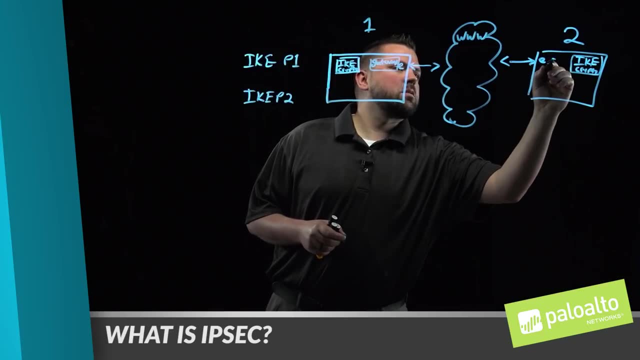 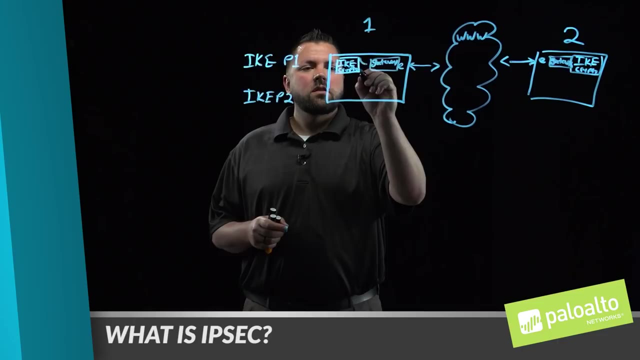 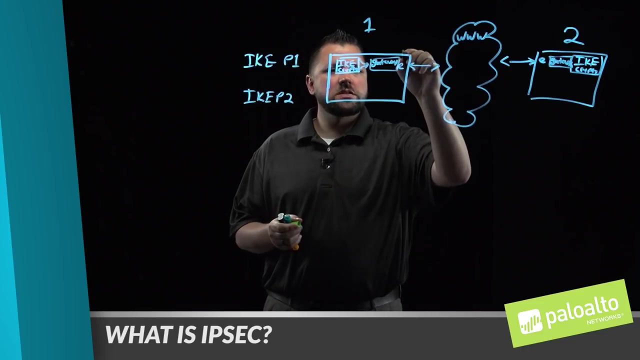 other is going to say: Then you establish a gateway And this is how the two peers get identified with another. The ikeCryptoSettings feed into the gateway and communication between the two starts out, as I said earlier, in ikePhase1, where the two sites first identify. 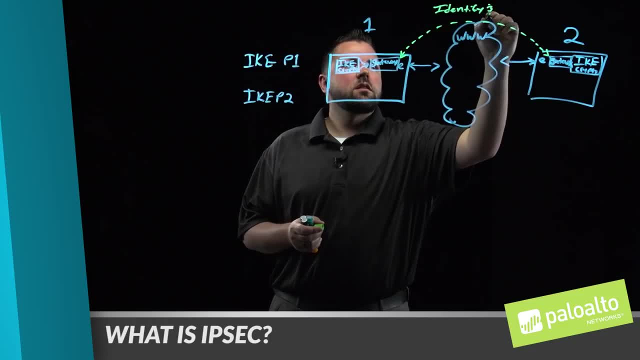 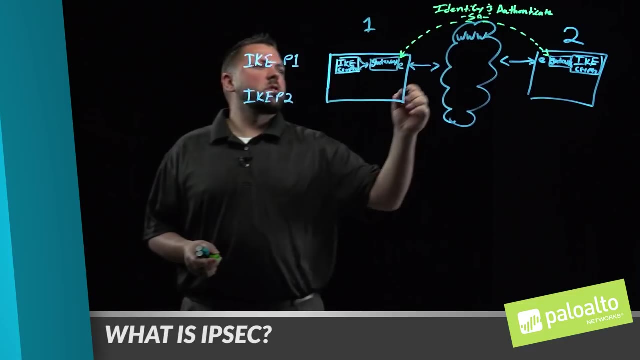 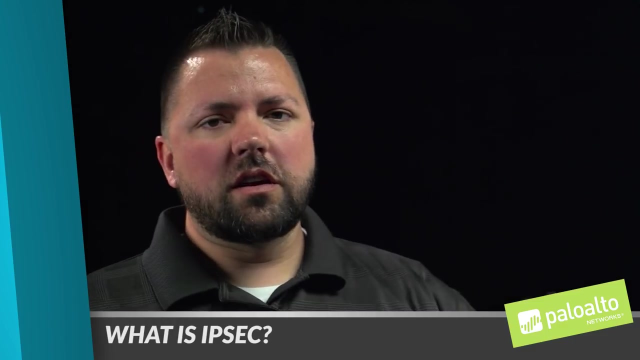 Okay, And then you authenticate each other and authenticate and establish what we call a security association. When the two gateways establish communications with each other, this communication all happens over UDP port 500.. The settings that go into the ikePhase1 cryptographic profile can be remembered. 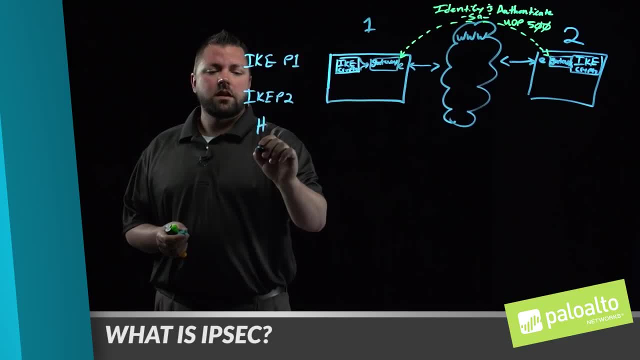 Okay, So let's do a couple of things before we get started. The first thing we need to do is find a word through a nice mnemonic H-A-G-L-E, haggle, or haggle, depending on where you're from. 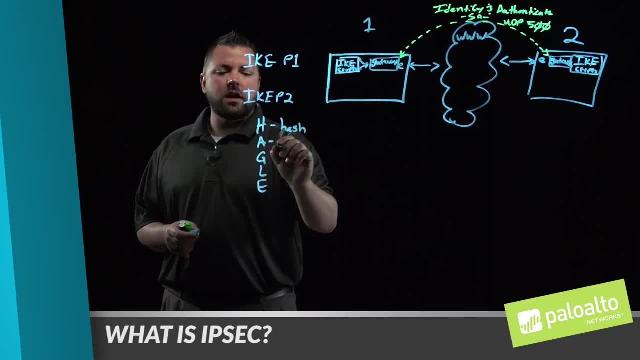 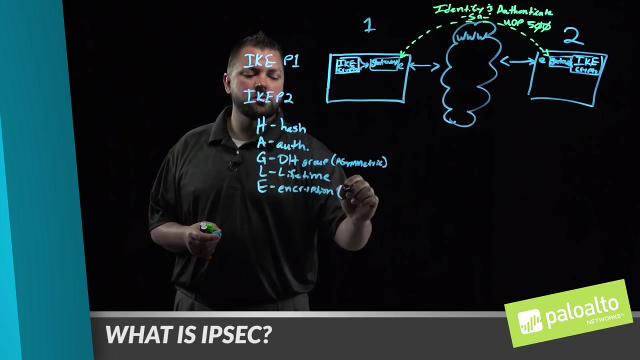 The first H is for hash, The A is authentication, The G- this is going to be your Diffie-Hellman group, and think of this as your asymmetric encryption key pair. Then there's a lifetime- Okay. And then, lastly, encryption, and this is going to be your symmetric or bulk data transport. 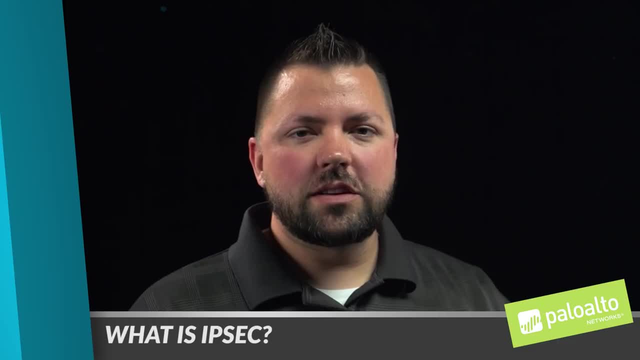 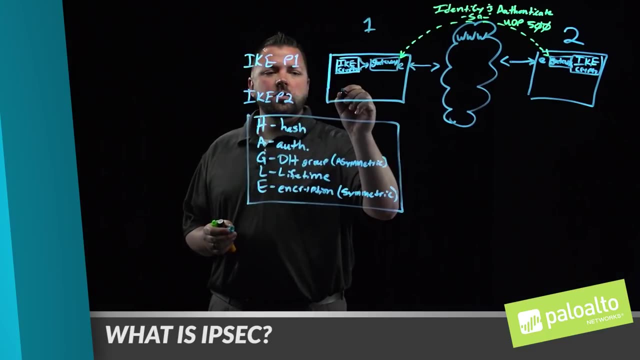 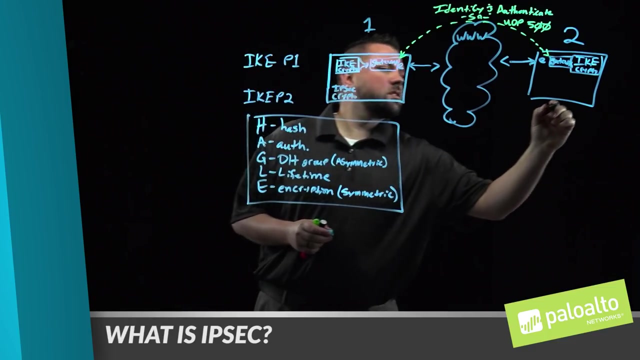 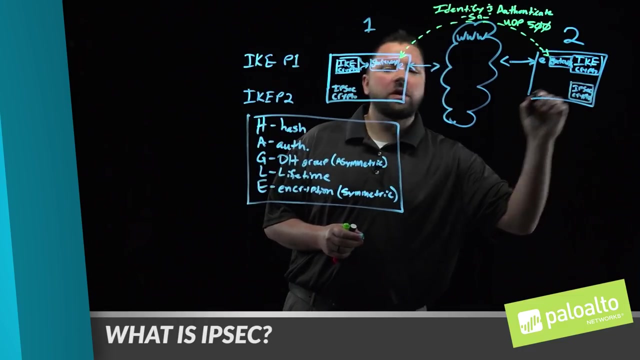 encryption. Now that the two peers have identified each other and authenticated with each other, they're ready to move into IKE phase two. In IKE phase two, we have what we'll call IPsec or IP security crypto settings on both sides. These settings must also match on both peers. 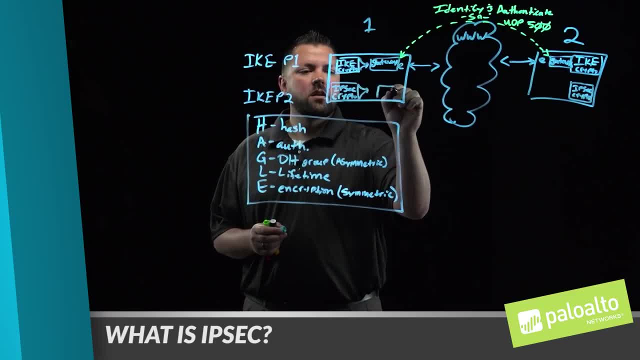 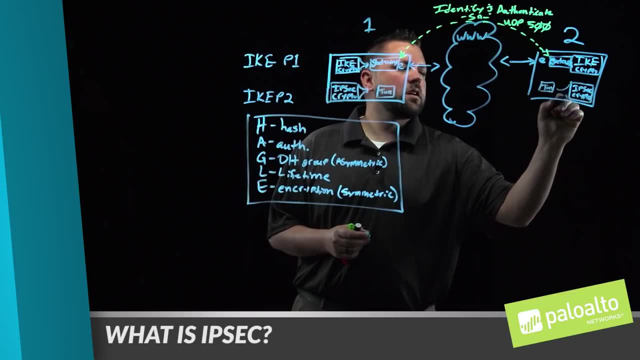 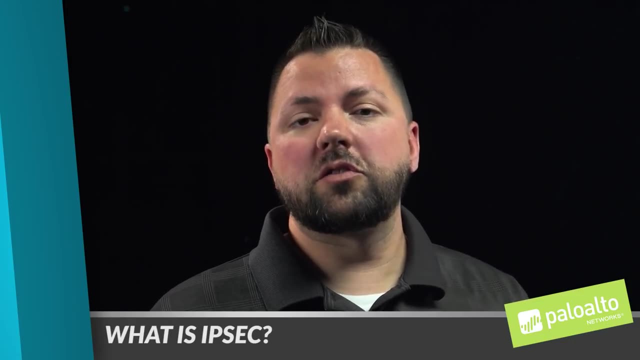 These settings then feed into the behavior of a tunnel interface. This is a logical interface in the firewall or router And between these two tunnel interfaces our symmetric encryption traffic or symmetrically encrypted traffic will traverse. Now that we have our two tunnel interfaces and their cryptographic settings are feeding, 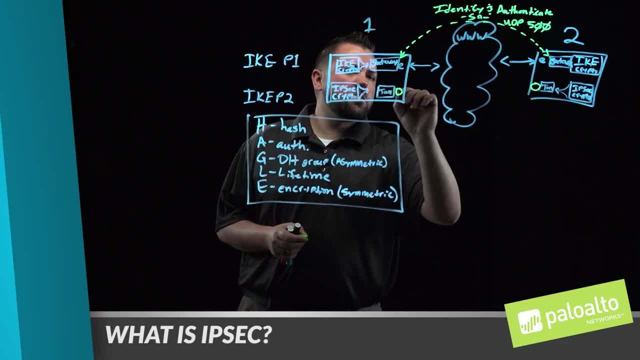 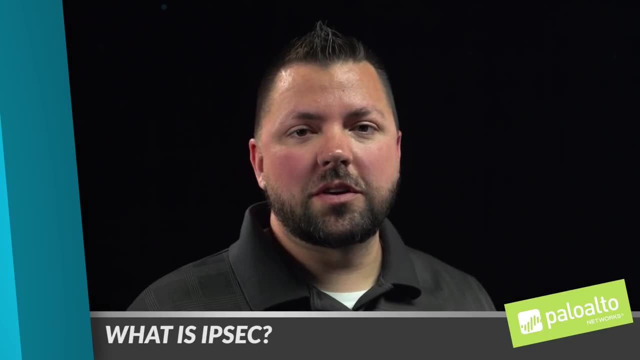 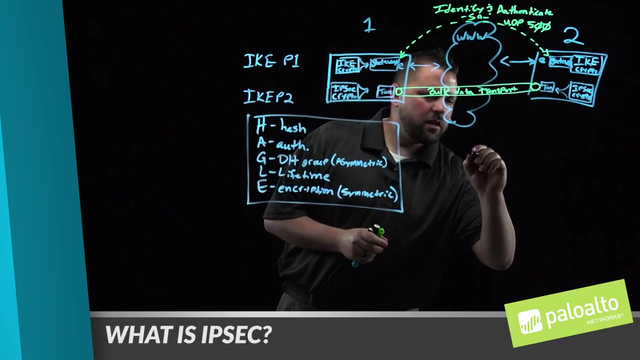 into the tunnel. we establish secured communications through a logical tunnel And this is going to be your bulk data transport And this is going to be IP protocol 50.. If you want to look at the traffic from start to finish, we're going to go ahead and do. 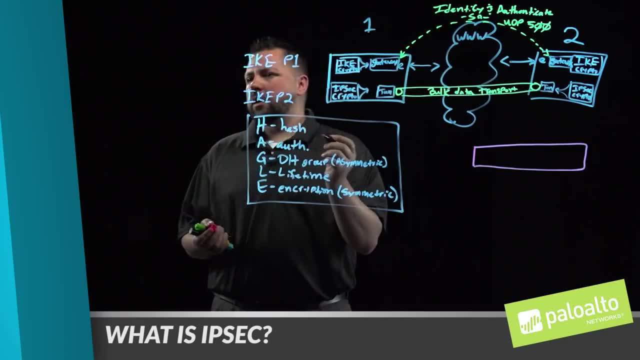 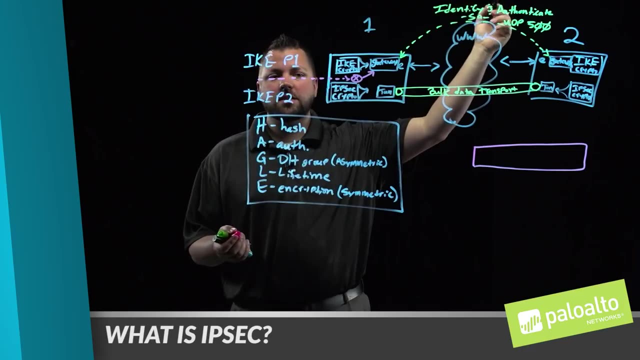 that We're going to start out with our original traffic. as it comes into the firewall or router, It's going to hit a router routing table and a decision is going to be made on whether it should go through the gateway and traverse through to the internet in clear text or 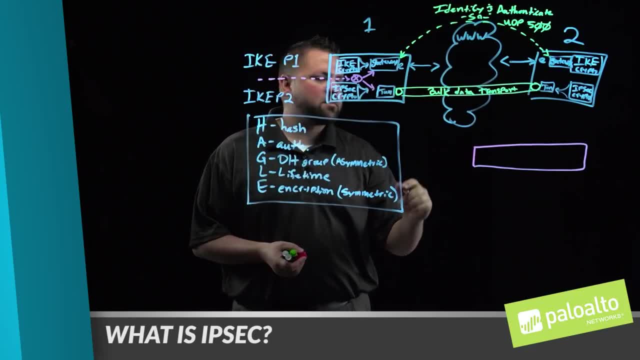 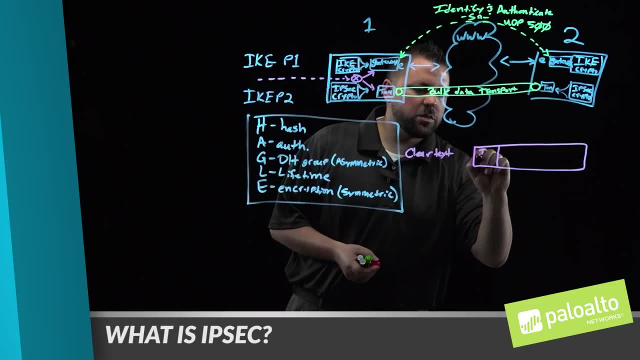 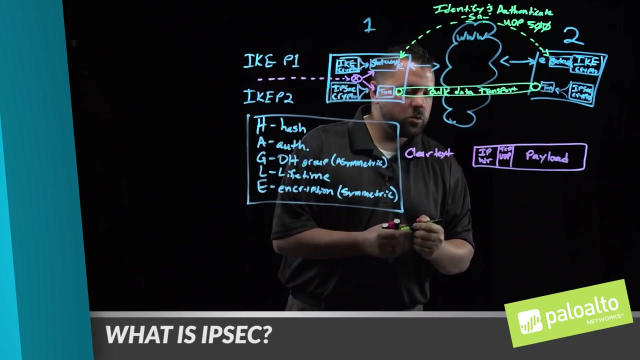 if it needs to go down to the tunnel interface and be encrypted. So your normal clear text traffic is going to have an IP header. It's going to have a TCP and UDP header or UDP header and then some payload. When this traffic gets encrypted, it can be encrypted in one of two modes. 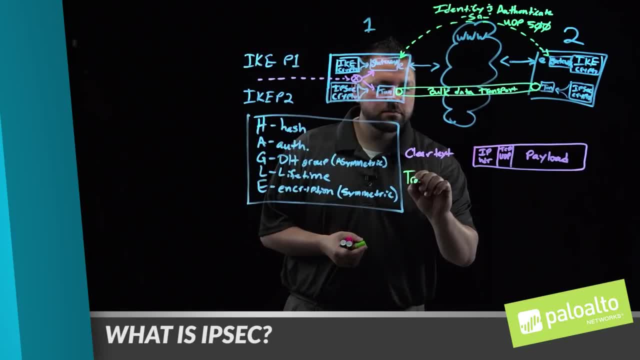 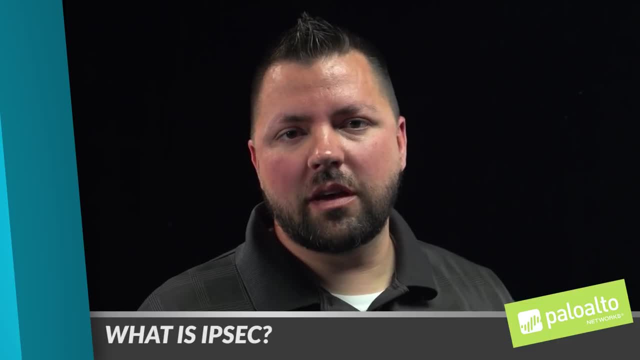 Our first mode we're going to call transport mode. Transport mode isn't the most popular for IPsec VPN tunnels, simply because the original IP header isn't in the tunnel. It's going to have a TCP and UDP header. It's encrypted. 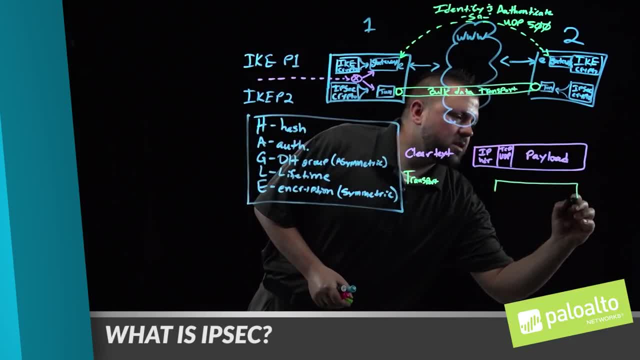 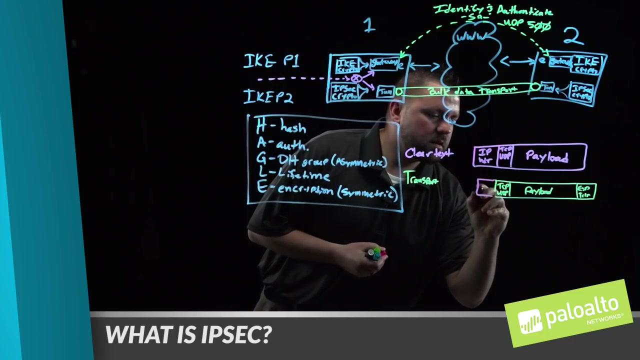 So let's see how that looks. The original TCP and UDP headers are encrypted, as well as the payload, And we add on a new ESP trailer for encapsulating security payload. Unencrypted is an ESP header. Unencrypted is an ESP header. 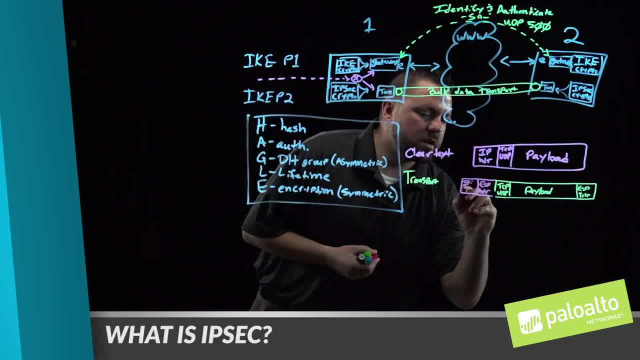 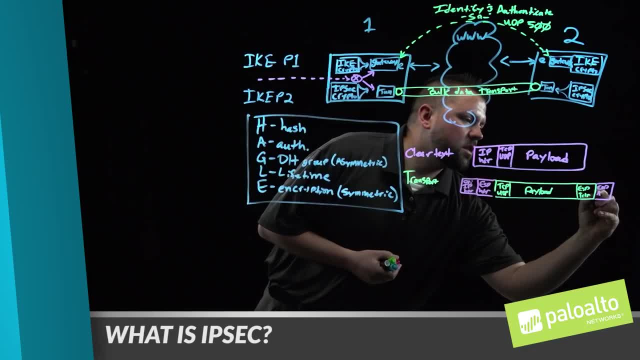 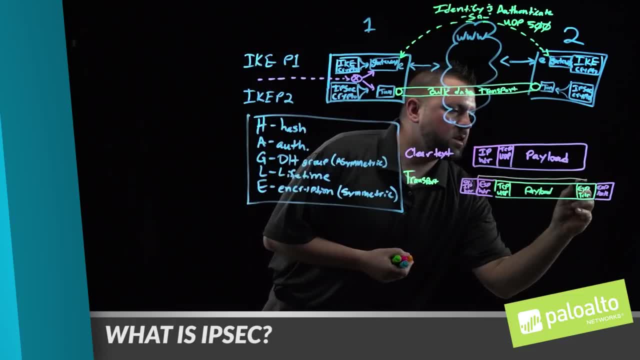 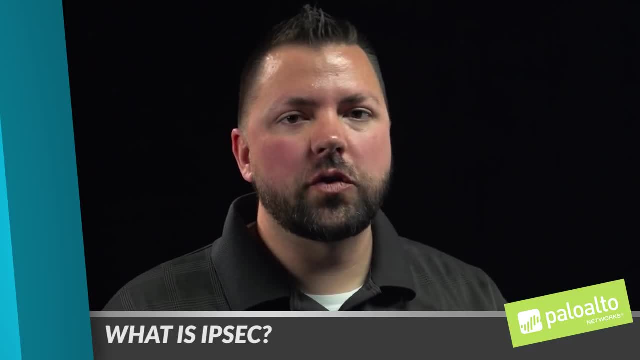 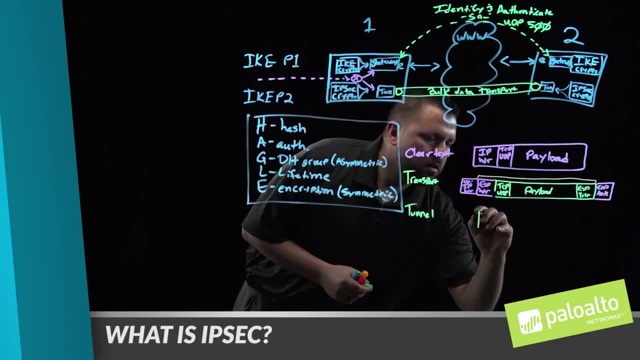 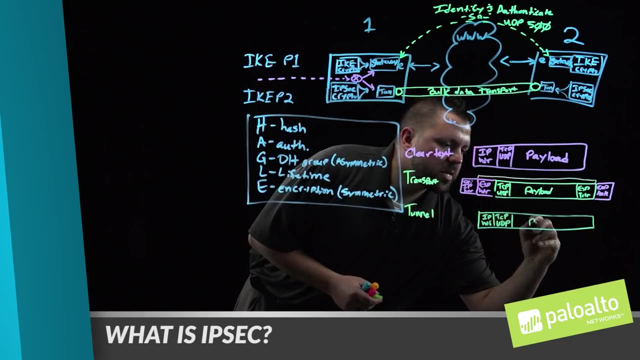 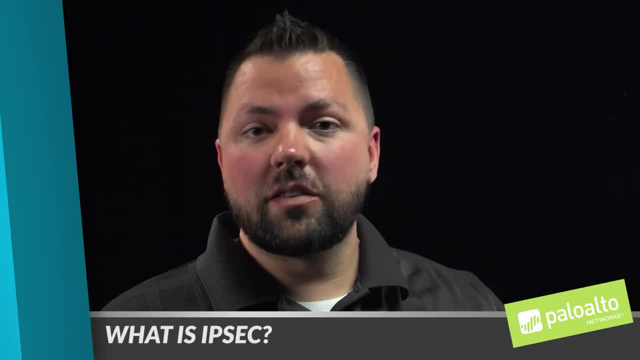 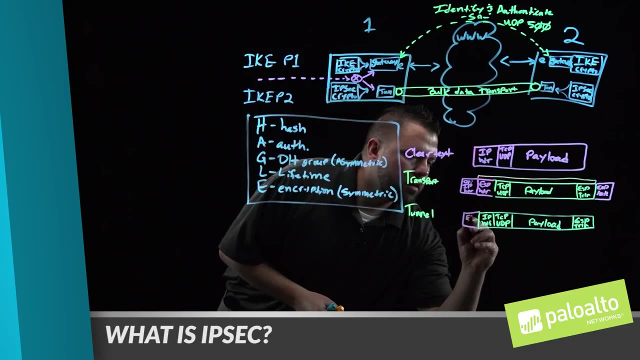 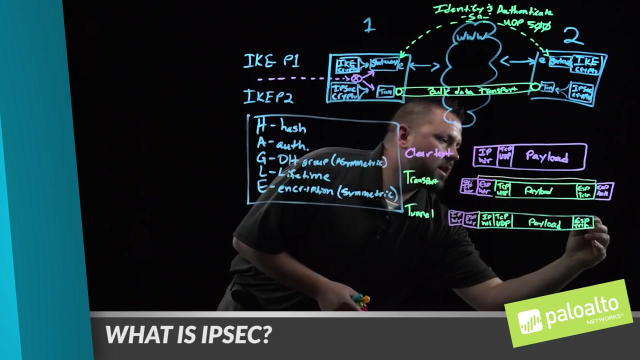 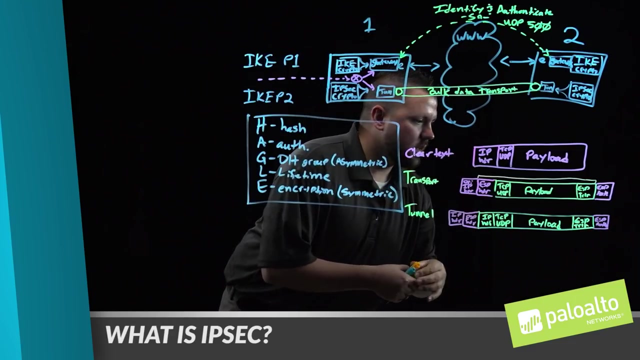 and as before with transport mode, the ESP header is unencrypted, and now we add a new IP header And our new IP header. And then, lastly, we have our ESP auth, And that auth trailer contains a hash of everything, including the ESP header. back to the ESP trailer. 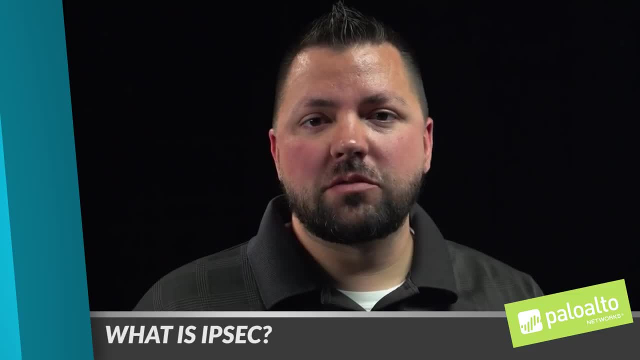 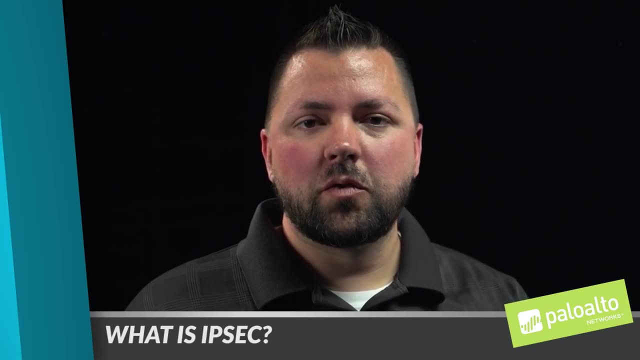 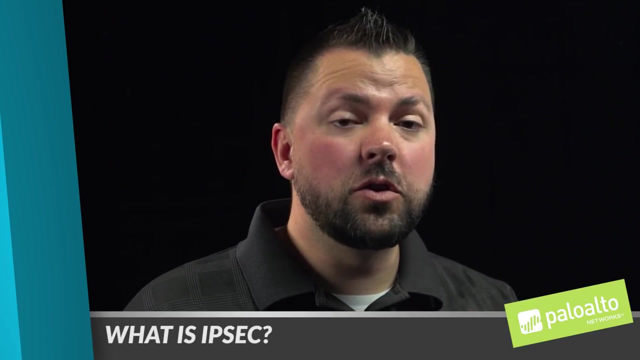 Now, sometimes an ISP could have a network address translation boundary somewhere in between the two sites, And so in order to get through NAT we have to turn on a new feature for tunnel mode called NAT traversal, And all that does is add a new UDP header right behind the new IP header, so that that 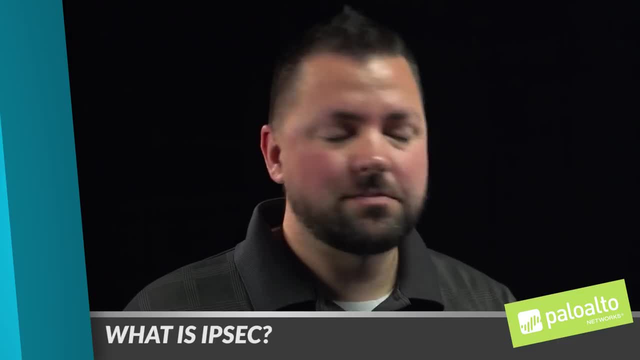 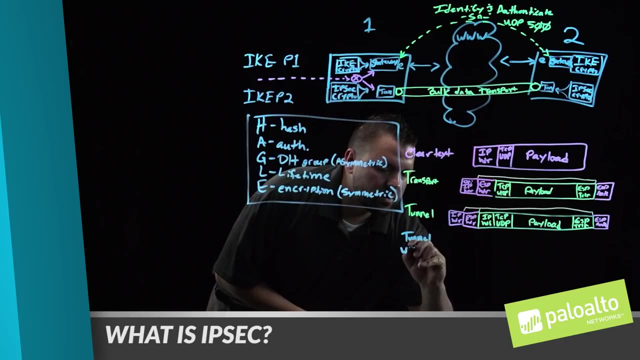 UDP header can translate between routers, So we're going to add tunnel mode with NAT traversal, And the way it will look is our new IP header. we have our UDP header and then our ESP header. This UDP header will be used across port 4500..